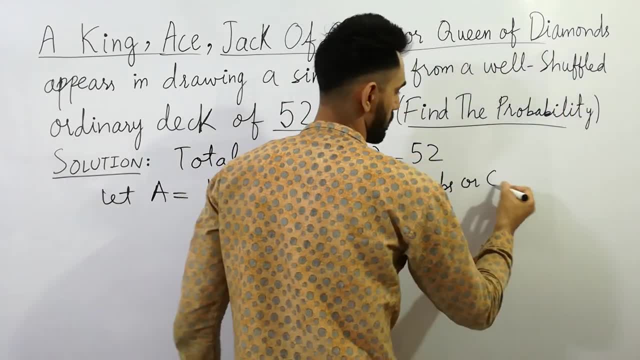 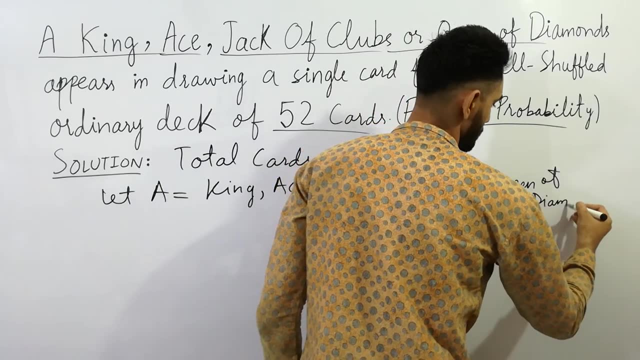 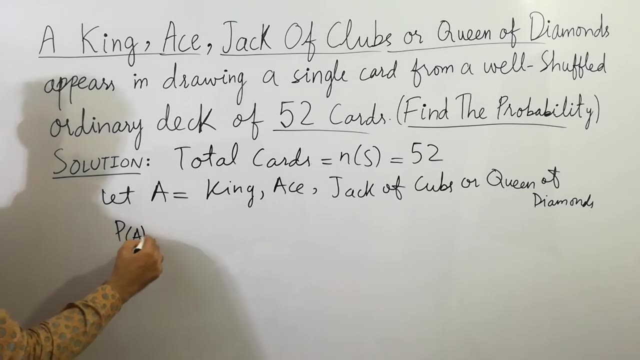 Or queen of diamonds or queen of diamonds. You have to find the frivolity of a. What is the frivolity of a? You know that frivolity of a is always equal to number in a divided by number in sample space. You can easily get rid of it. 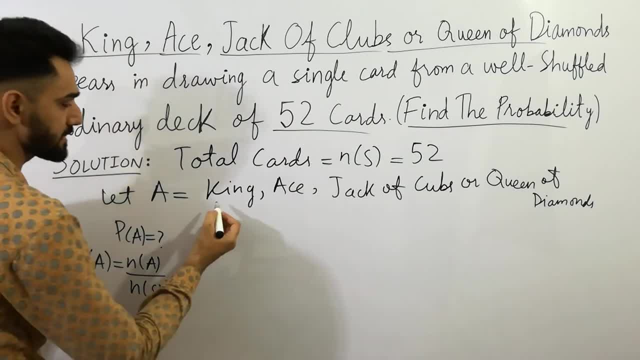 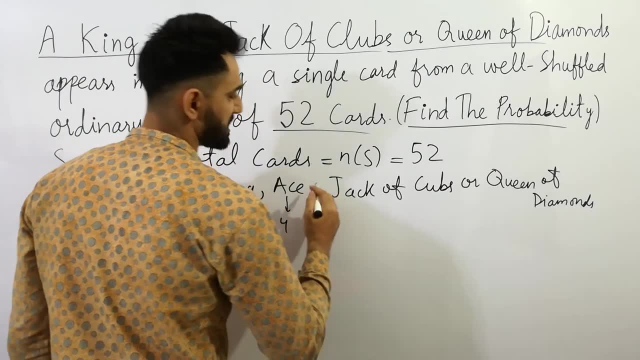 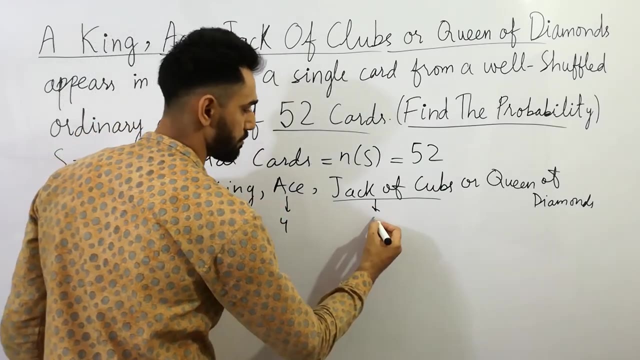 So here a is given here king. What are king? King is always for mustard diamond and ass is always for an ass. and jack of clubs is clubs is 13,, but jack of clubs is always 1, so put here 1, an ass. 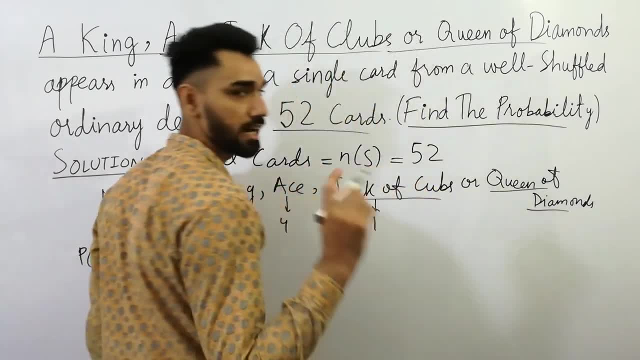 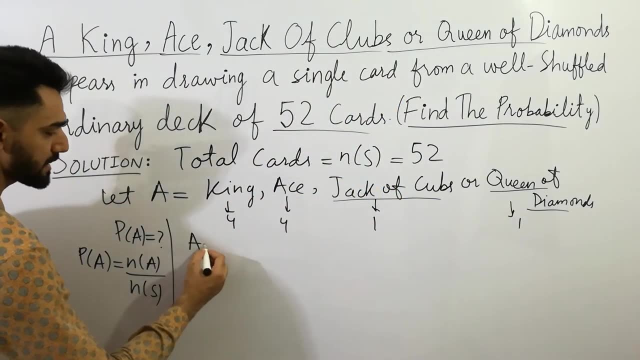 Diamonds are 13,, but queen of diamonds are always 1, so write here 1,. so here you can easily calculate the value of a. a is equal to 1.. So here a is equal to 4, plus 4, plus 1, plus 1.. 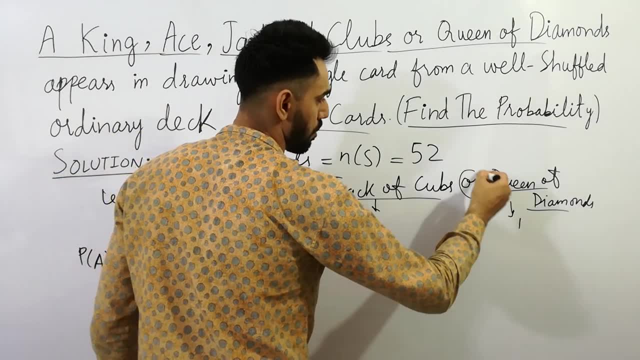 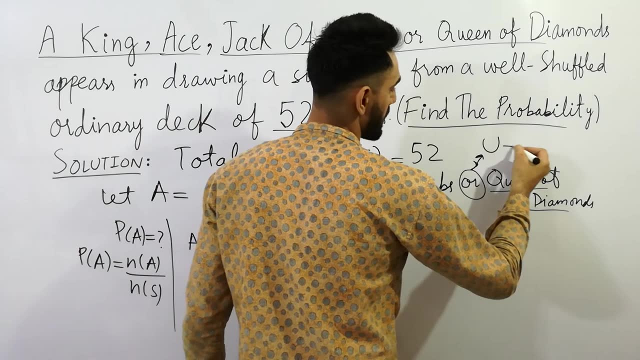 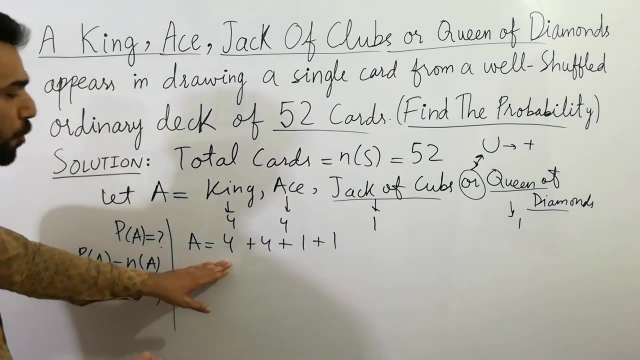 Because you know that this is the sign of or. Or represents the union. you know that Or represents the union and union always represents the addition. So here this is the law of addition applied here. So here, 4 plus 4 plus 1 plus 1, we'll get here 4 for 8,, 9,, 10.. 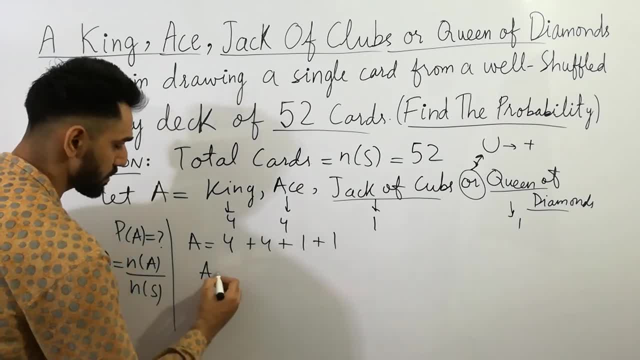 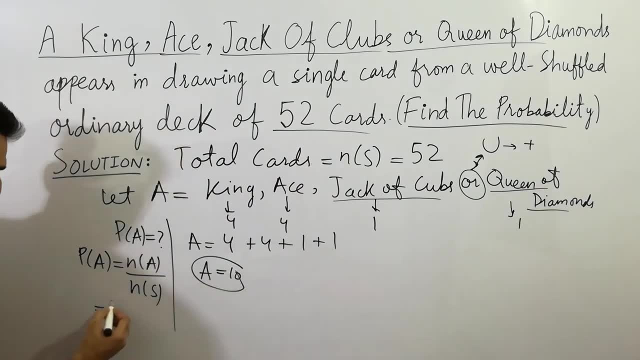 So here is the value. here a is equal to 10.. So here you can easily calculate the value. now The value of a as a number in a are here: 10 divided by total 갓's are 52.. So the value is given here: 2, 1 is a 2,, 2, 5 is a 10.. 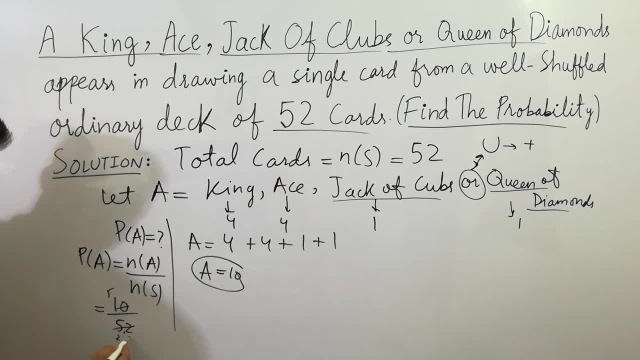 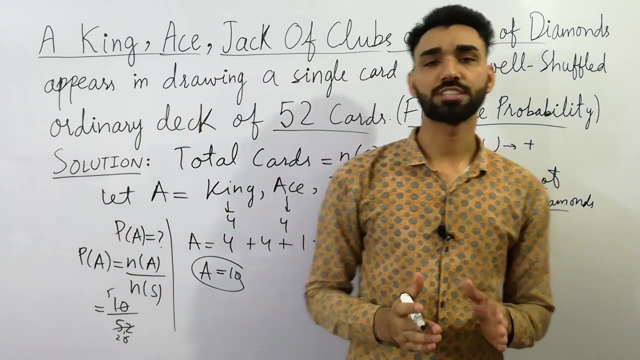 Two, twos are 4 and when you long more, there are two sixes are 12.. So here the probability of a. So the probability of a. we have calculated here 5 over 26, so this is the probability of this question. thanks for watching this video also. 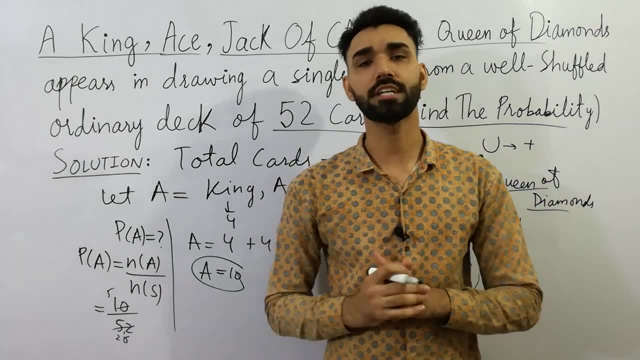 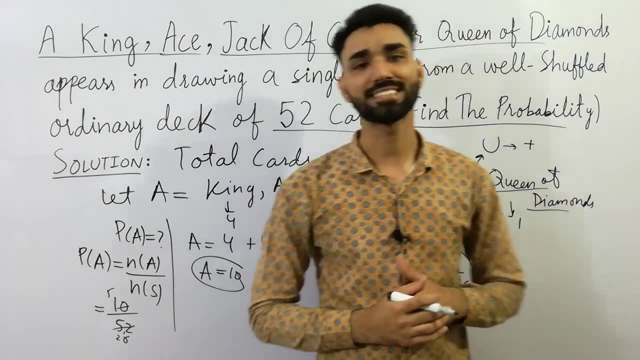 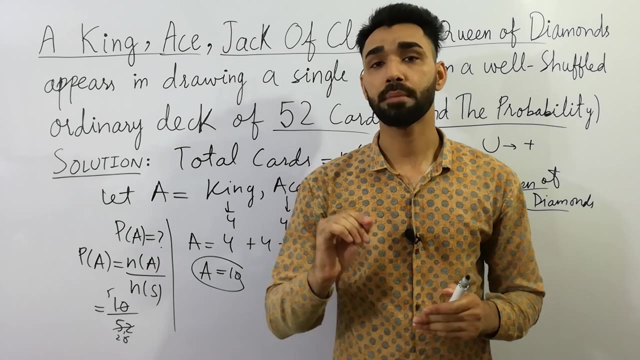 share this lecture with your classmates and friends so that they also have a benefit of it, and also visit the playlist of this channel to learn more and more about statistics and probability and mathematics. and don't forget to like and subscribe this video and must press bell icon button to get the notification of my new lecture. goodbye.